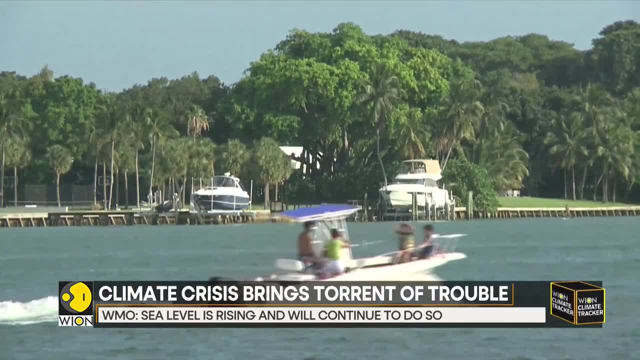 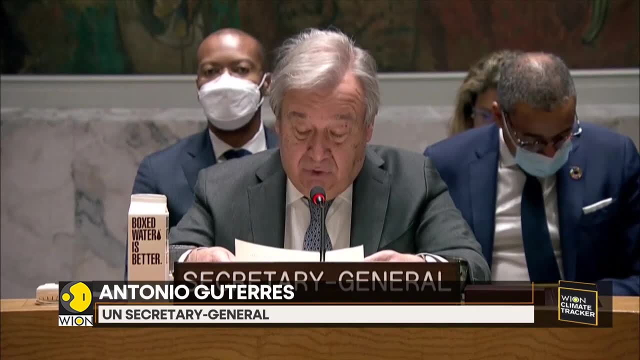 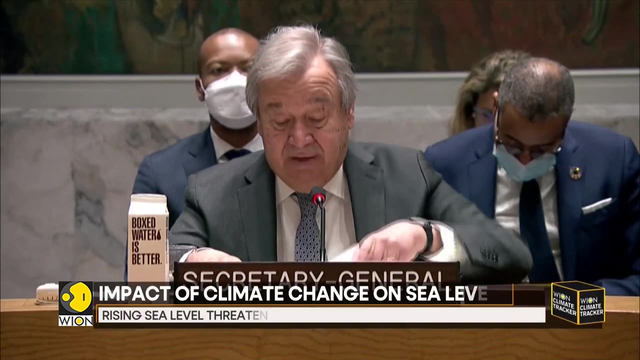 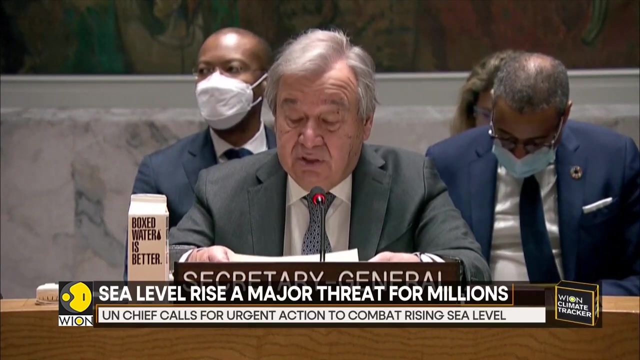 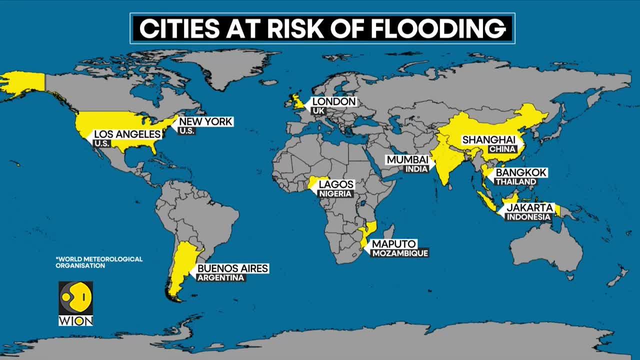 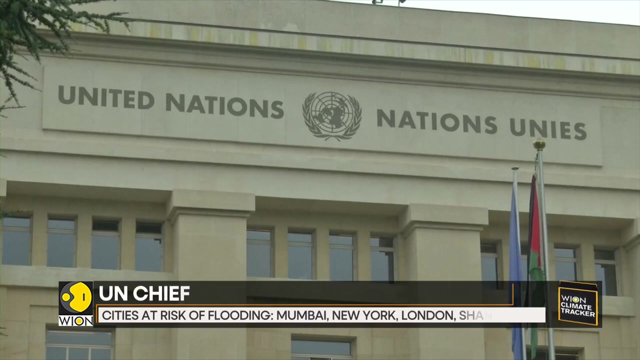 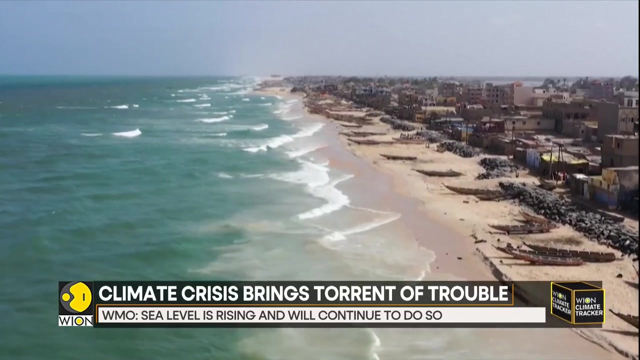 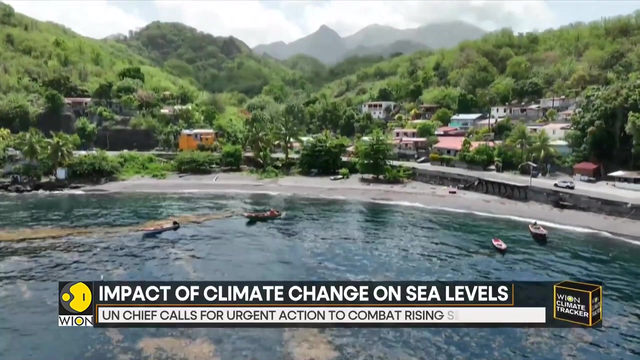 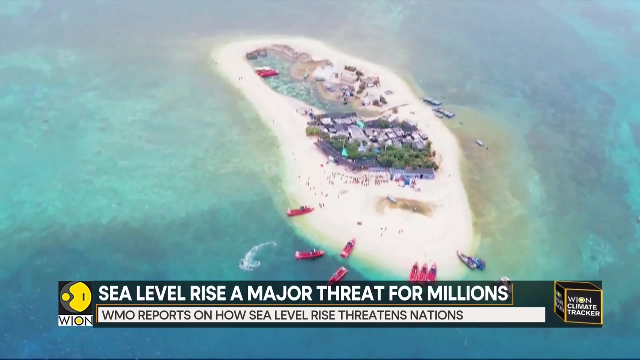 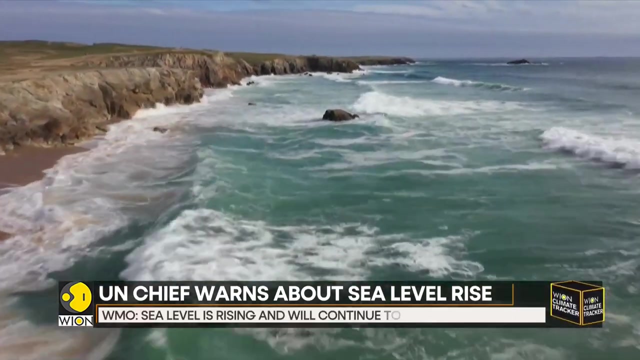 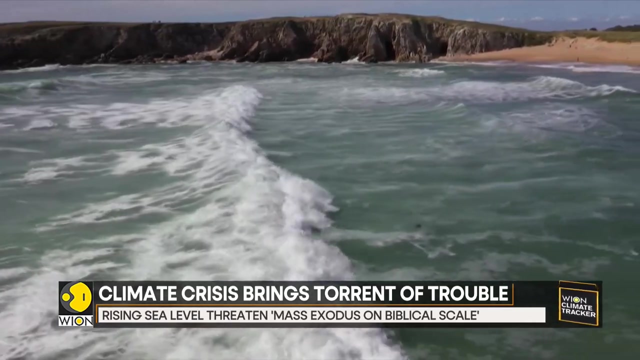 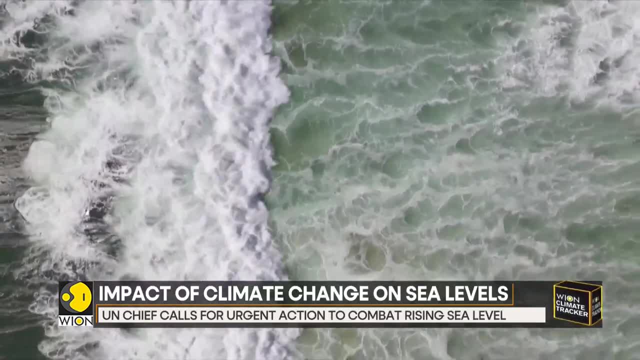 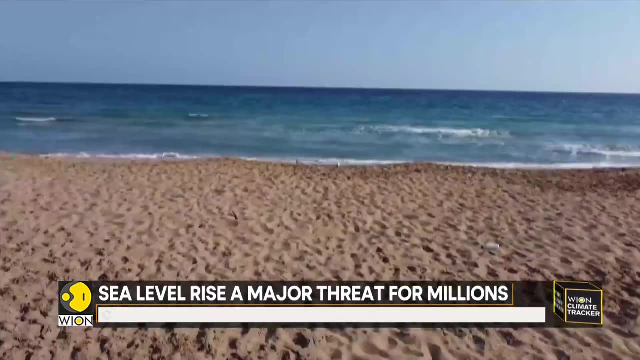 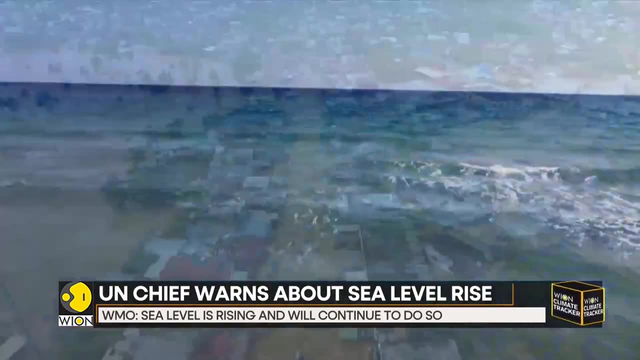 to warm up by just another 2°C in comparison with the pre-industrial era, then those levels could actually rise by as much as 43cm by the year 2100.. But if it warms by about 3 or 4°C, then sea levels could rise by as much as 84cm And experts fear that continued. 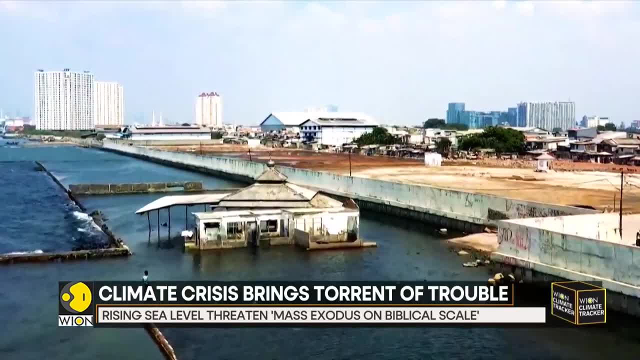 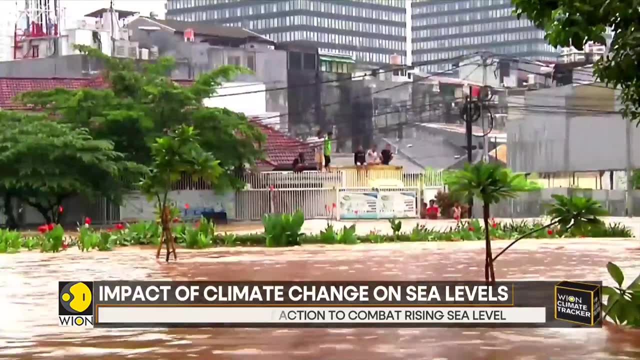 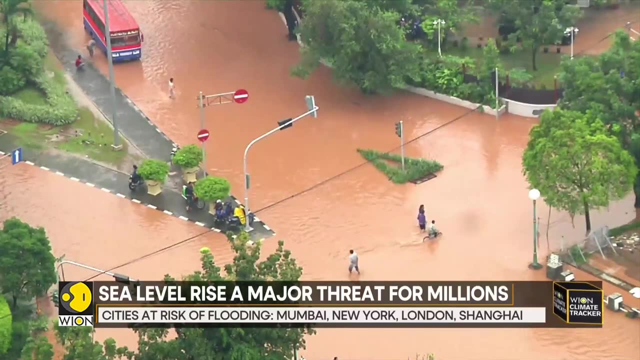 and accelerating sea level rise will encroach on coastal settlements and infrastructure and will commit the low-lying coastal ecosystems to submerge, which would cause the erosion of coastal ecosystems, will worsen the intensity of storm surges and flooding, and this can also lead to contamination of soil and groundwater with salt, further impacting food security. 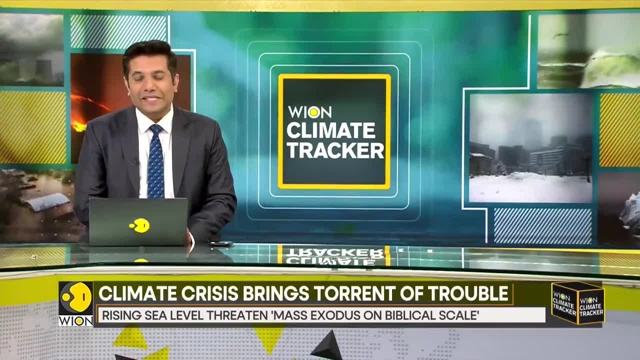 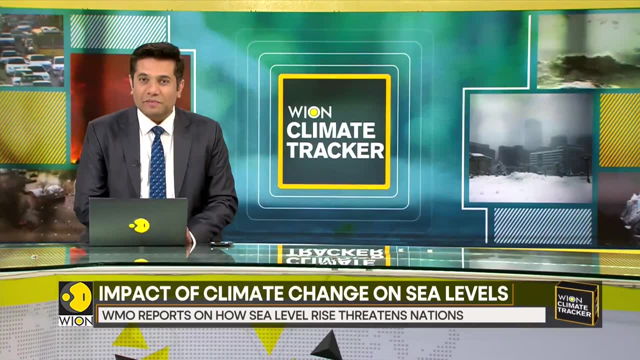 To give us more insights in terms of the rising sea levels and how this is likely to impact humanity in the next coming few years and decades. we're being joined in by Maggie Rodriguez, who's joining us from Parana in Brazil. Maggie is a science. 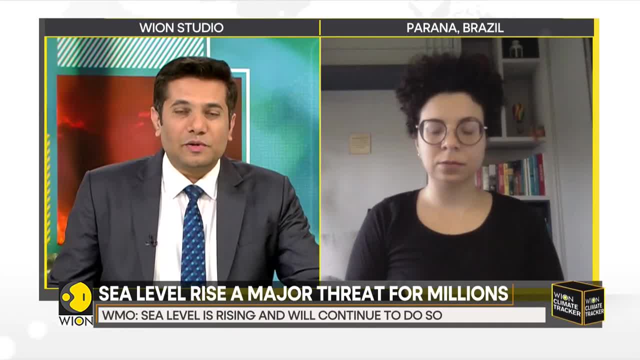 scientist at the University of Parana and she's going to tell us a little bit about the climate crisis and climate journalist who's joining us on this broadcast. Ms Rodriguez, thank you very much indeed for joining us on this broadcast And the 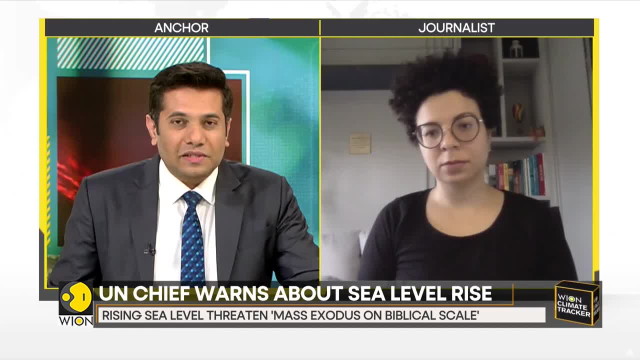 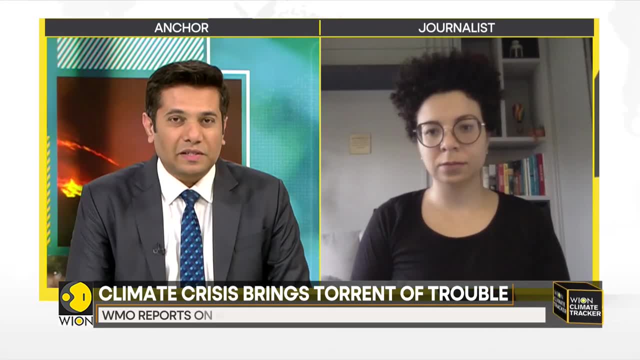 question that I want to ask you is: you know, this is a dire warning that has been sounded by the United Nations Secretary-General, António Guterres, where he said that at least about a billion people could be impacted because of the rising sea levels. Is there something? 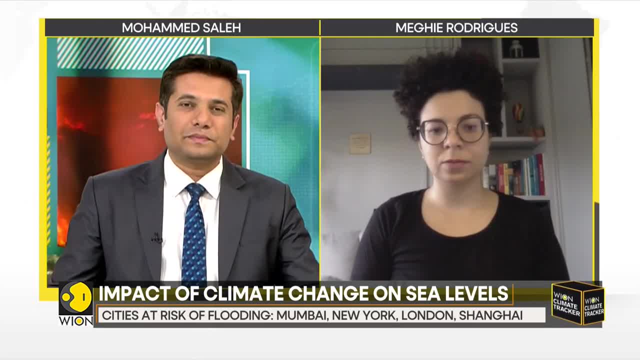 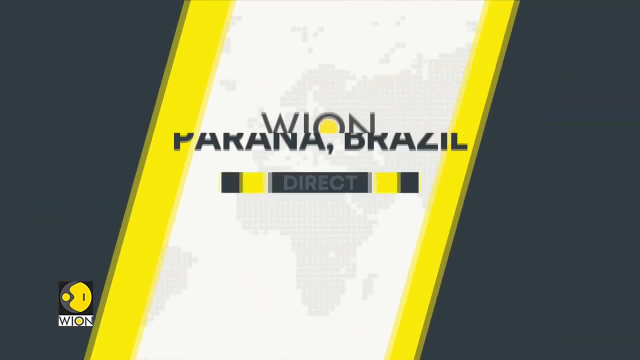 that nations can actually do to reverse this Sure. So, first of all, thank you for having me here. Good evening to all. I'm so happy to be here. Good evening to everyone watching this show right now. Yes, there's a lot that. 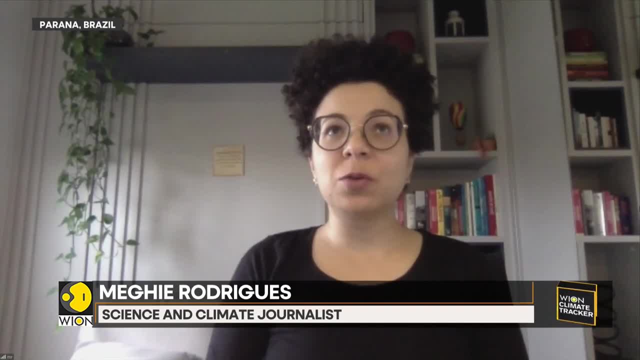 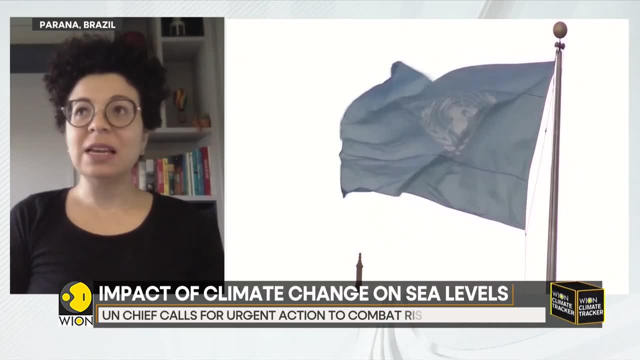 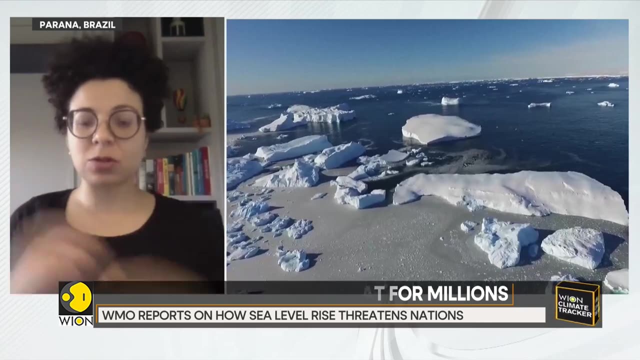 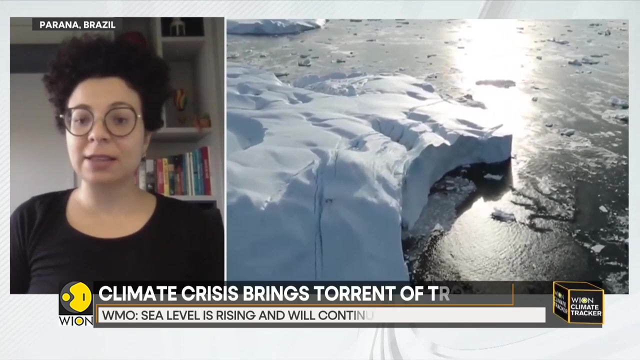 can be done. First of all, greenhouse gas emissions can be cut, And we all know that absorption, like the technologies for absorption and burial, so to say, of greenhouse gases, is not- I mean, they are not- It's developed at a large scale yet, so we cannot count exactly on technological solutions. 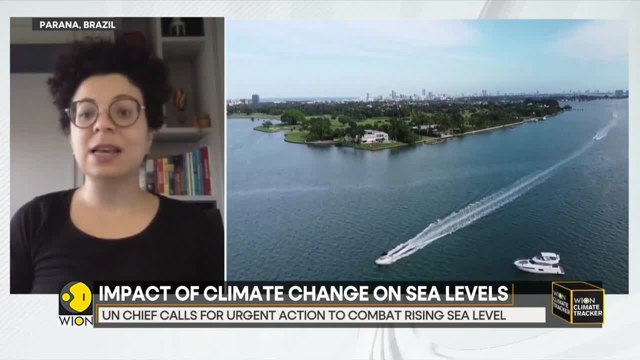 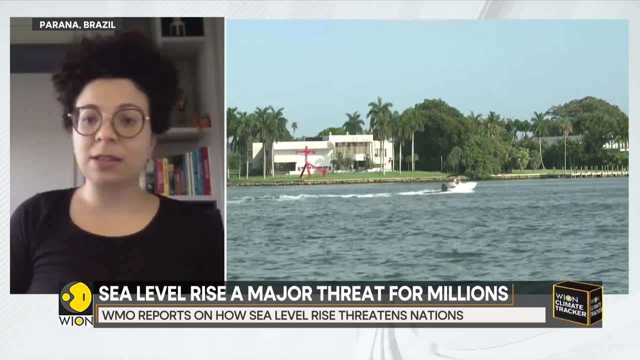 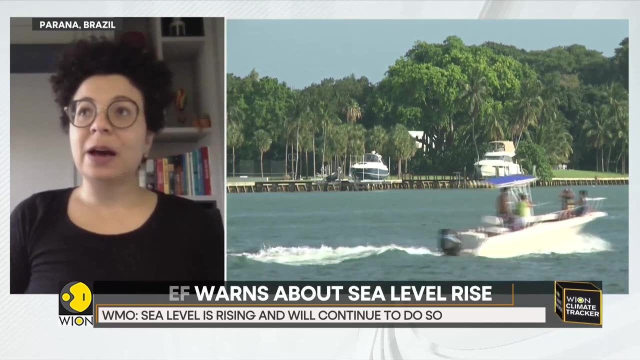 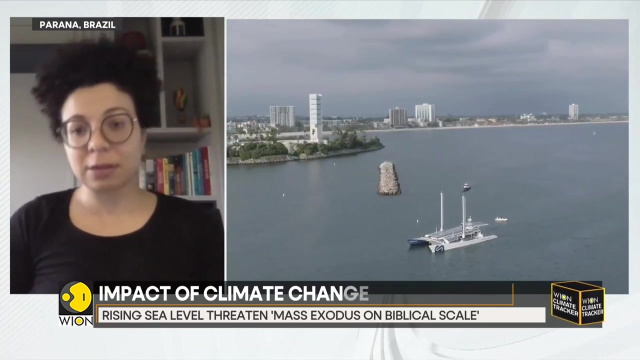 So the best solution is really to cut emissions as much as possible. And another thing that can be done- but it's not as developed as it should- is climate financing, especially the payment for low-lying countries and poor countries. So you know the payment for low-lying countries, you know for damage, like the payment for 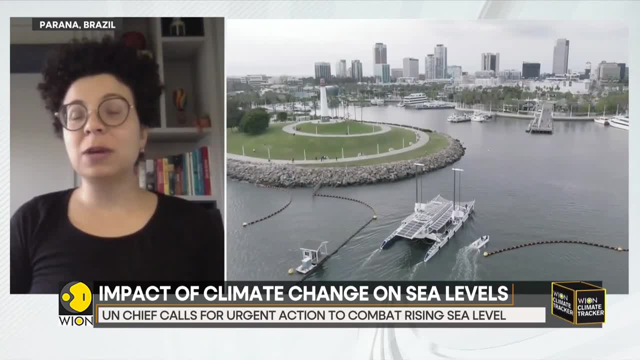 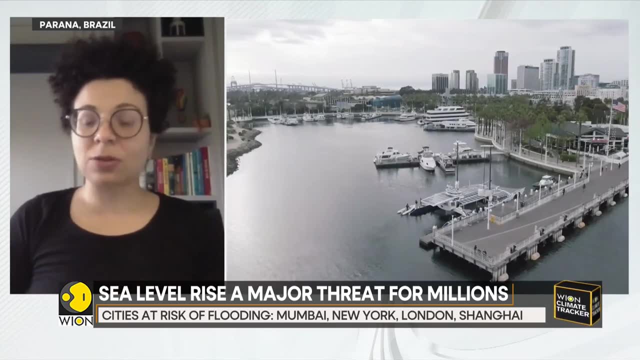 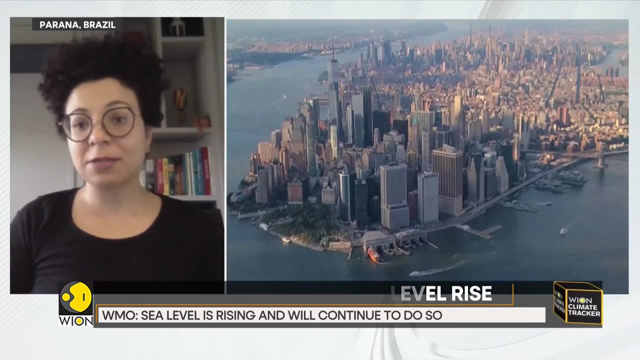 damage and also the financing for mitigation and adaptation policies which have been talked about in the last many, you know, COP negotiations that we have seen but have not been in place yet. Now, at this point, you know, as we speak, leaders around the world, they all agree to. 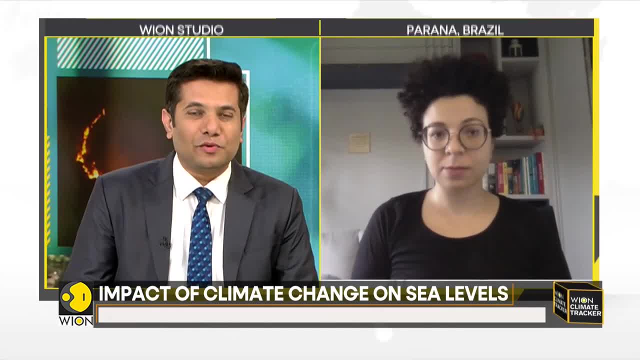 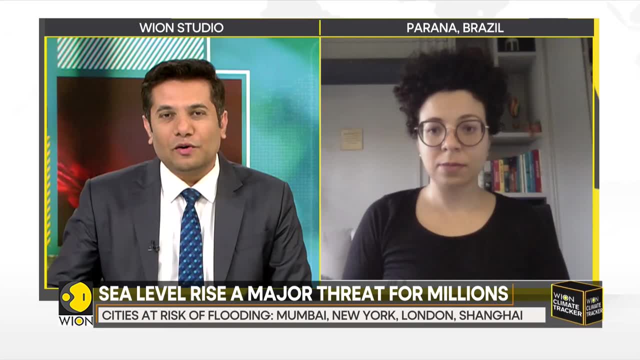 the fact that climate change needs to be stopped. They're also putting in legislations. They want to have what are known as these zero-carbon economies, But most of the targets are by the year 2050 or by the year 2060.. 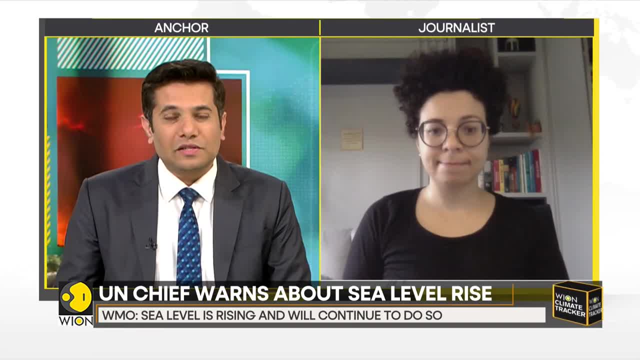 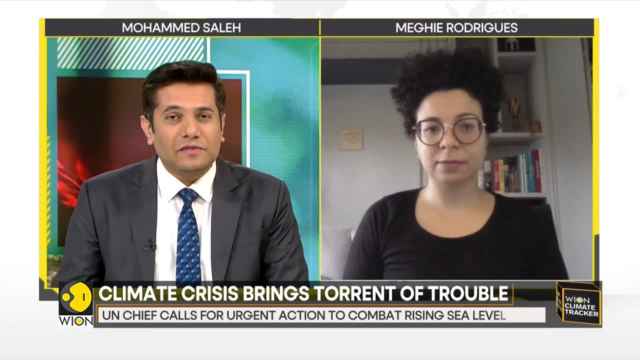 That is when most of the countries are likely to meet these targets. With that being the case, do you think realistically? you know we can put in place the mechanisms that are needed to actually reverse the process of adding extra carbon into the atmosphere. 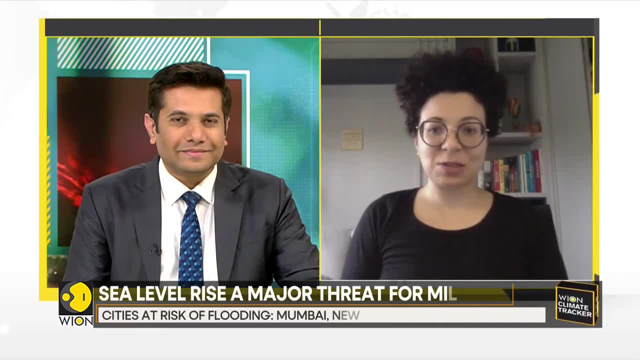 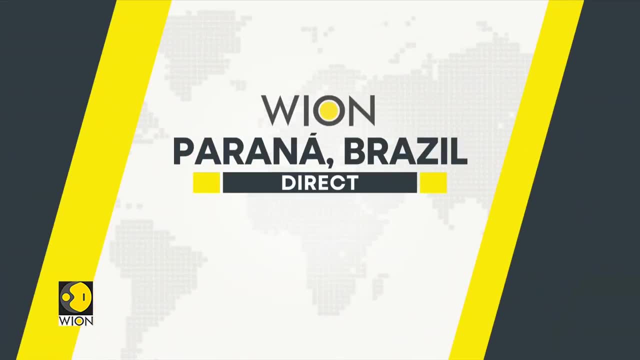 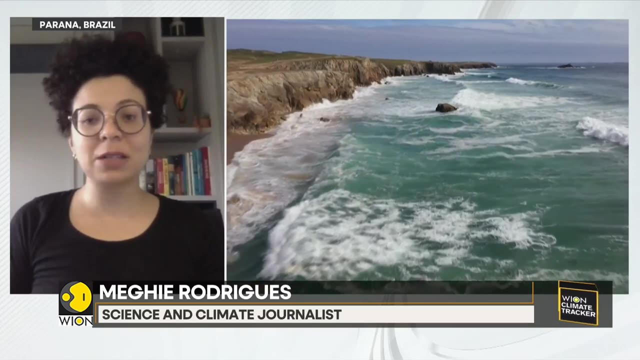 Realistically. yes, Absolutely Yes, we can, But I don't know if there's enough political and economical will to do so before a catastrophe. So yeah, we would need much more engagement and much more real, you know, political and. 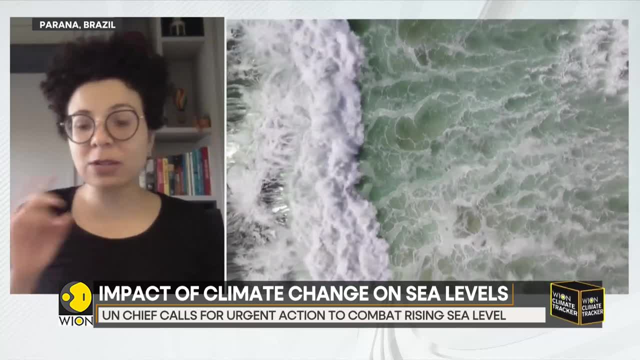 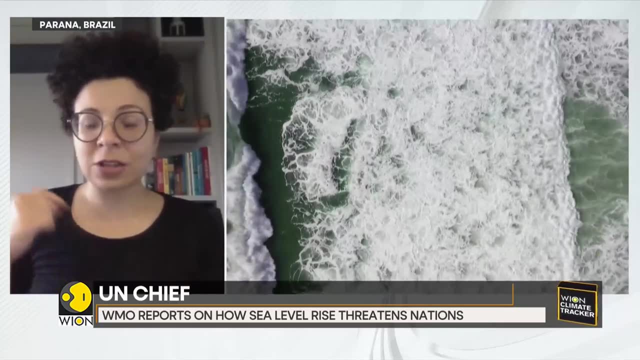 economical will to do that Right, You know. just to give a few numbers, if I may, Yeah, Yeah, Yeah. So you know the US and other US government agencies just last year they talked about 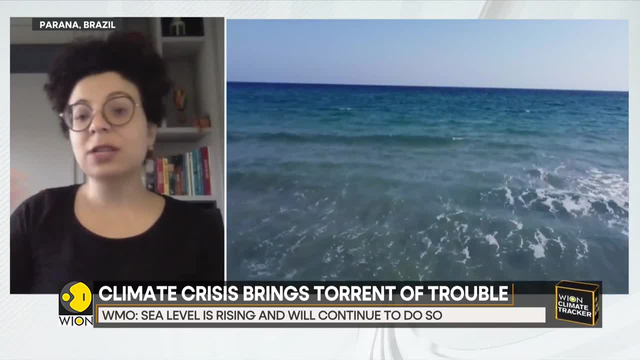 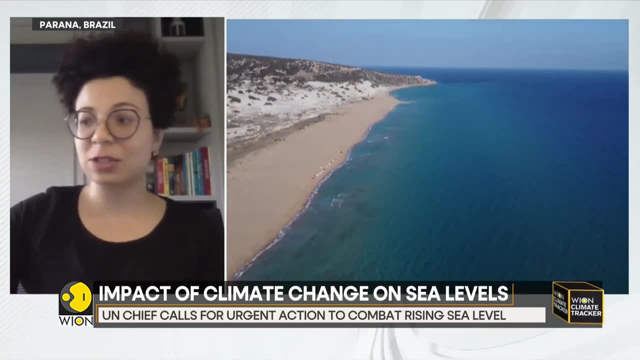 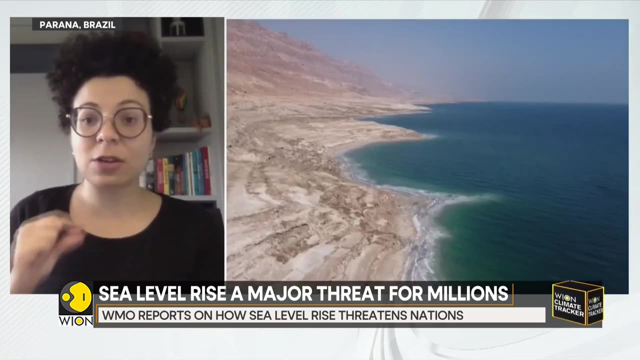 some numbers of sea level rise until 2050, which is just three decades away. So it's not 2100.. It's not from here to you know two centuries, It's just three decades away, Because sea level rise is not going to happen at the same rate and at the same you know. 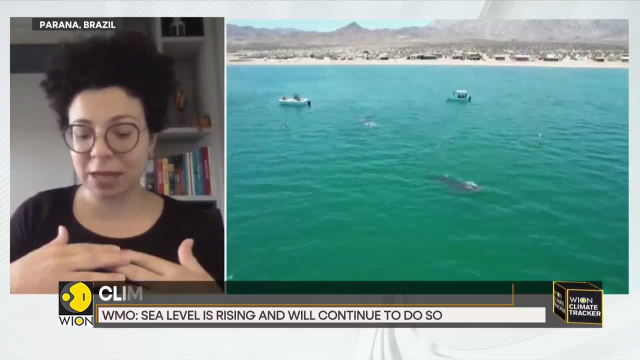 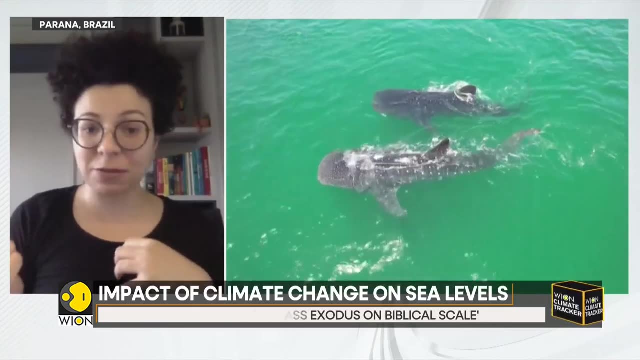 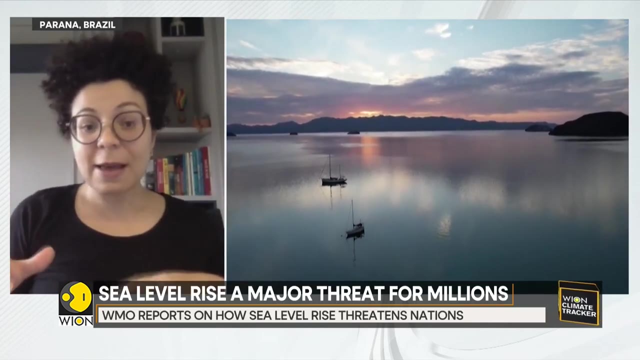 with the same price. It's not going to happen at the same. how can I say it's not going to rise? the same for all countries? That's true. So until 2050, in the Pacific coast, we're going to have from 10 to 20 centimeters rise. 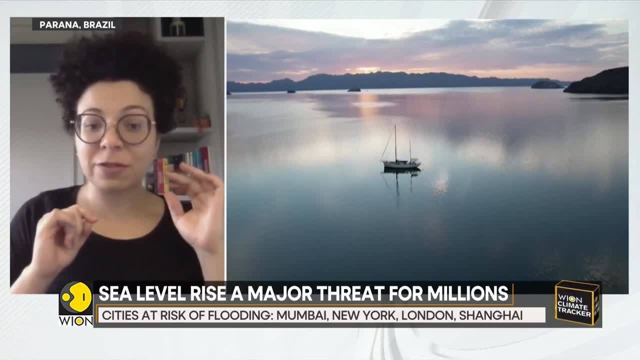 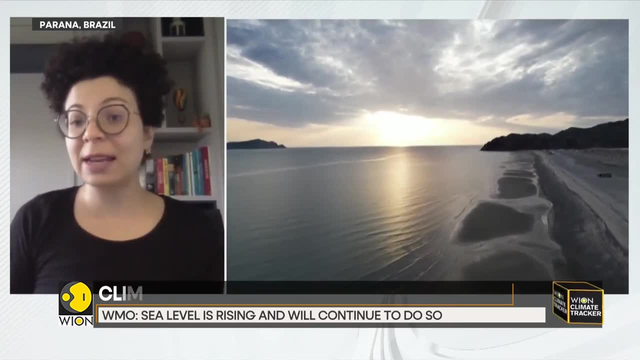 But on the Gulf, for example, we're going to see from 35 to 46. So it's almost half a meter of sea level rise. if we don't do anything, You know, it's just three decades. So it's just three decades away from now. 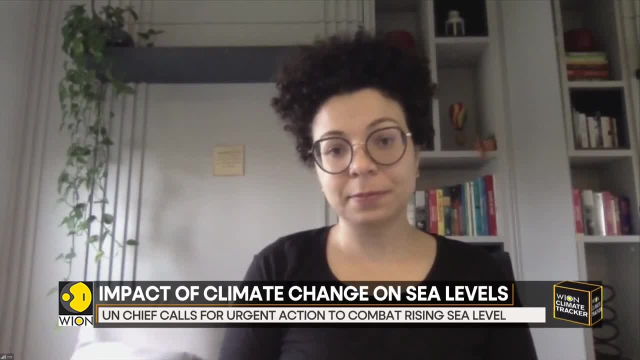 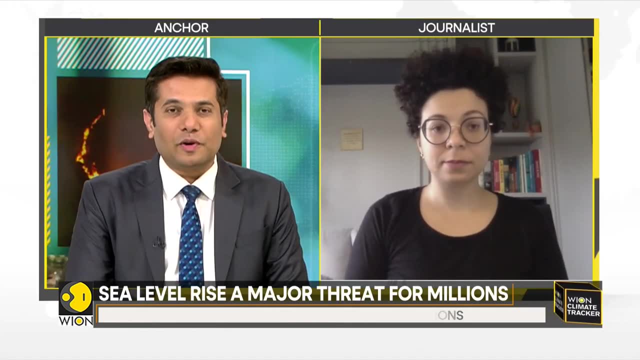 Right, That's. that's absolutely well summed up. I think that, of course, it remains the crux of this issue: Will the nations actually find the political will to address the problem of climate change? Thank you very much indeed, Ms Rodriguez, for joining us from Brazil and getting us. 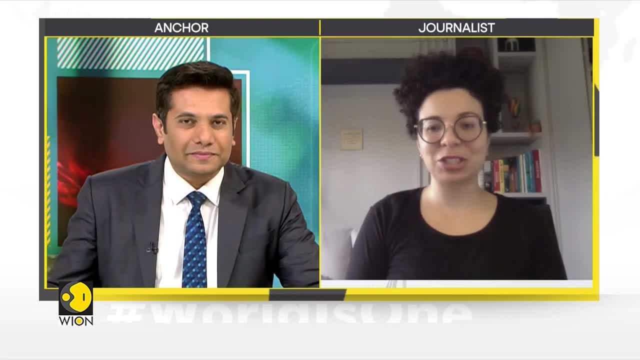 all those insights there, Thank you, Thank you very much. Beyond is now available in your country. Download the app now and get all the news on the move.